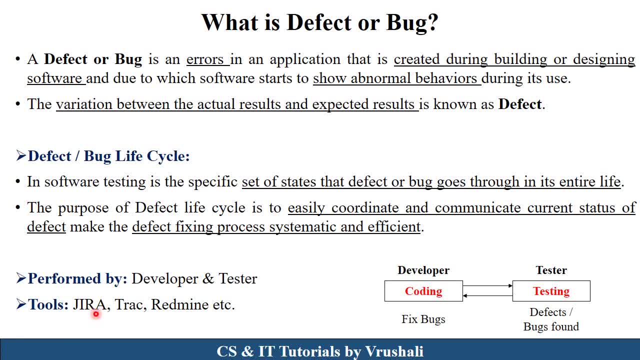 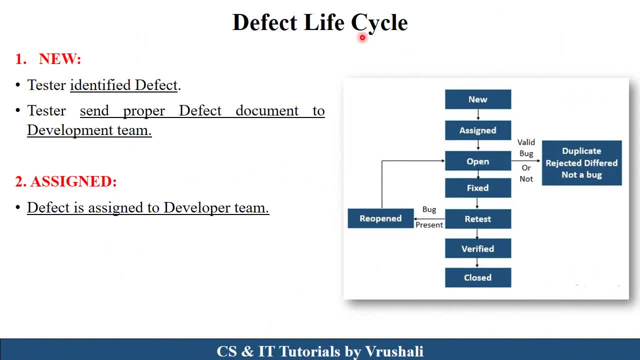 tester. For that purpose they use different tools like JIRA, TRAC, Redmine, etc. Now the next topic is defect life cycle. As per your exam point of view, this question and this diagram is important. The first state in defect life cycle, that is, new state In testing phase. 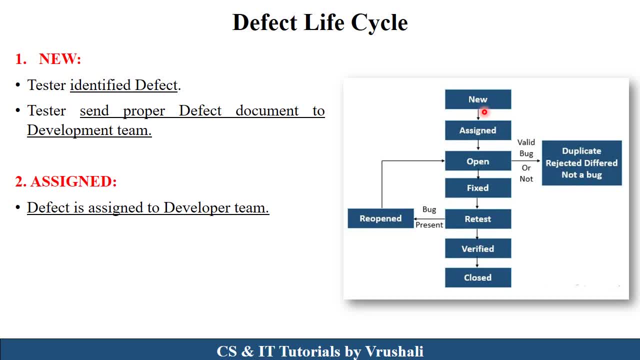 tester identified defects or bugs in particular project, Then they send this particular defects to the developer team for solving purpose. This is called as new state. After that there is a assigned state Here. all the defects are assigned to the developer team for solving purpose. 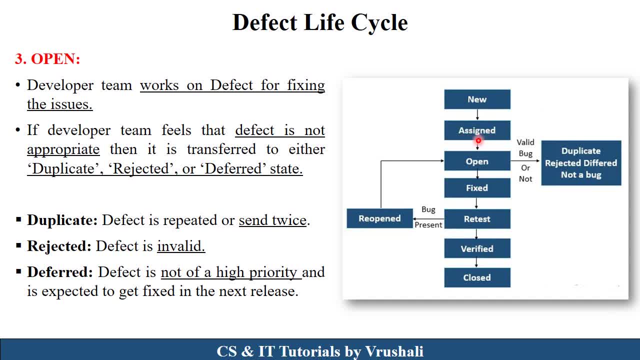 Now, after assign all the defects to the developer, there is a open state Here. developer open a particular defect and change the state. After that, the developer assigns all the defects to the developer team, and so on, until the developer team decides whether a defect is valid or invalid. 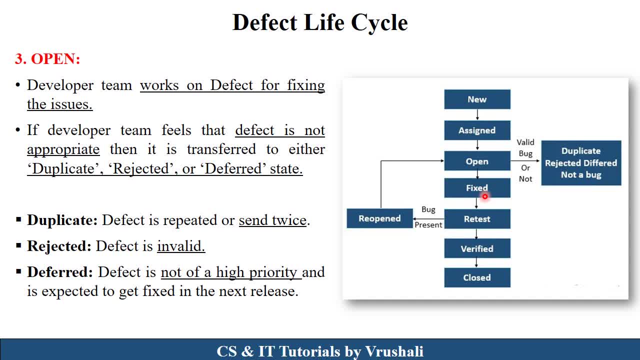 If particular defect is valid, then they move to next state, ie fixed state for solving purpose, But a particular defect is invalid At that time. they transfer those defect into 3 states, like duplicate, rejected and differed state. Suppose tester send same type of defect again to the developer, this is called duplicate state. 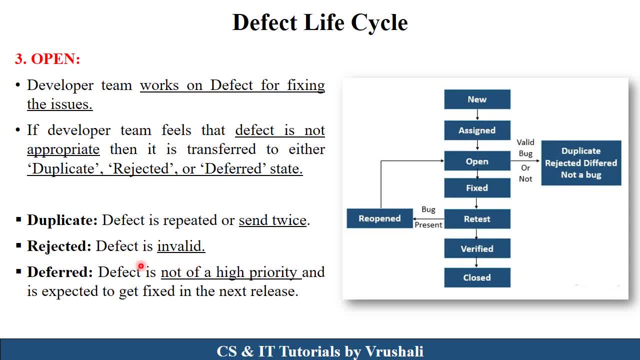 Suppose defect is invalid, ie rejected state, which is fifth stage, update, allono lan and third base. So each critical issue under states for death is published in debug' struct state and sometime defect is not as that high priority so you can solve those. 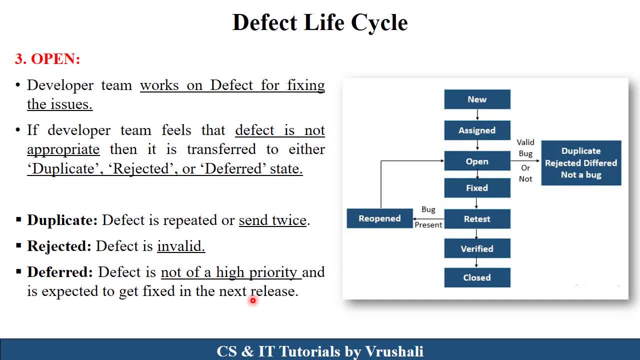 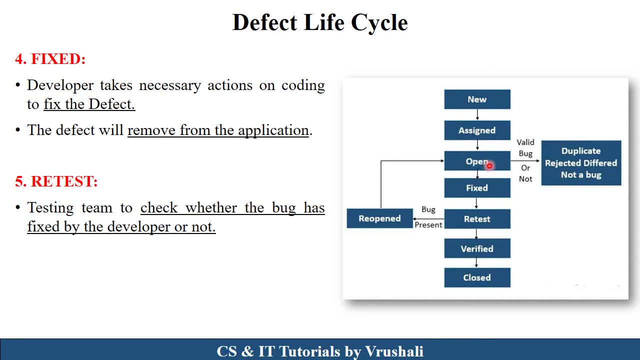 defect in next release and next version of particular software. this is called as deferred state. now, if a particular defect is valid, then they move to fixed state. here developer takes all the necessary actions to solve a particular defects, errors in particular project and they ensure that all the defects will. 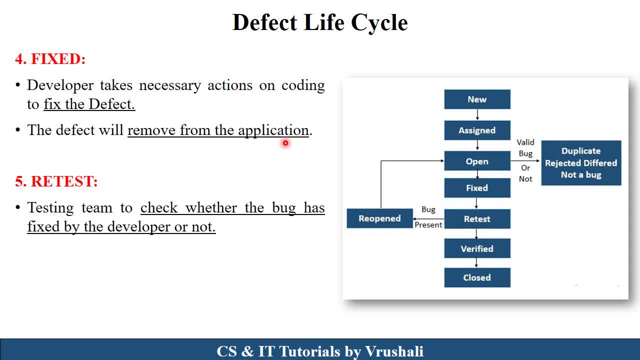 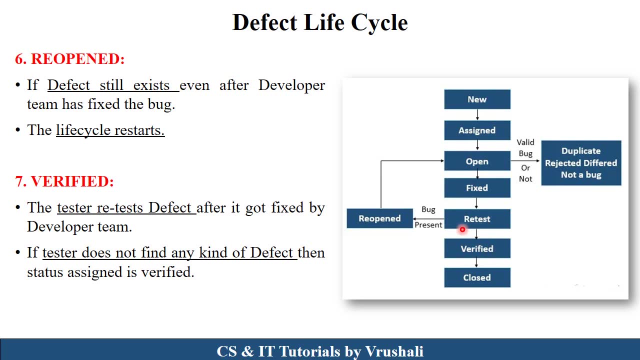 remove from particular project and they send this status to the tester. now the next one is retest. here testing team check that whether a particular defect has fixed by the developer or not. now in retest, suppose a particular defect is still present in particular project, then they move to reopen state this defect again sent to the developer.